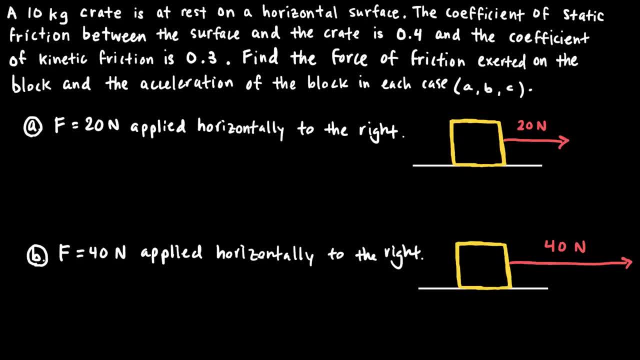 In this video I'm going to work out a simple example to help us better understand the difference between static and kinetic friction. A 10 kg crepe is at rest on a horizontal surface. The coefficient of static friction between the surface and the crepe is 0.4, and the coefficient of kinetic friction is 0.3.. 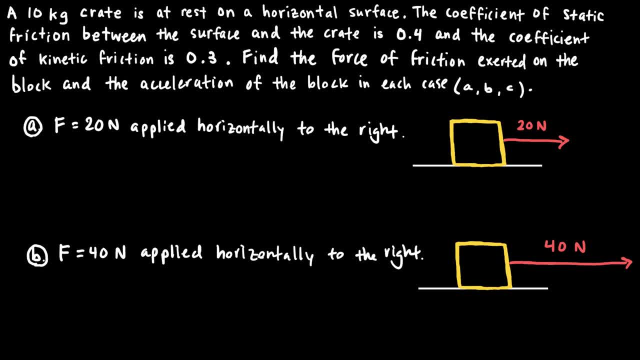 Find the force of friction exerted on the block and the acceleration of the block in each case. So I'll be looking at three different cases. Case A: a force of 20 N applied horizontally to the right. Case B: a force of 40 N applied horizontally to the right. 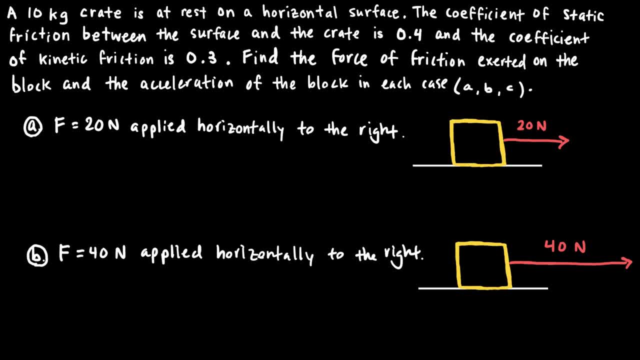 And then, eventually, we'll look at a case C where an 80 N force is applied at an angle above the horizontal. But let's start with part A. The first question you should ask yourself is, when dealing with either static or kinetic friction, is which one should you use? 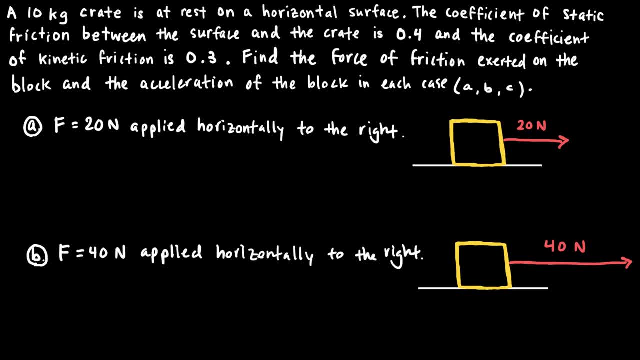 And the way that you would determine that is, you would need to see if the force that's being applied to the block is enough to make the block move. If the force that's being applied is greater than the maximum value of static friction, then the block would move, the block would accelerate. 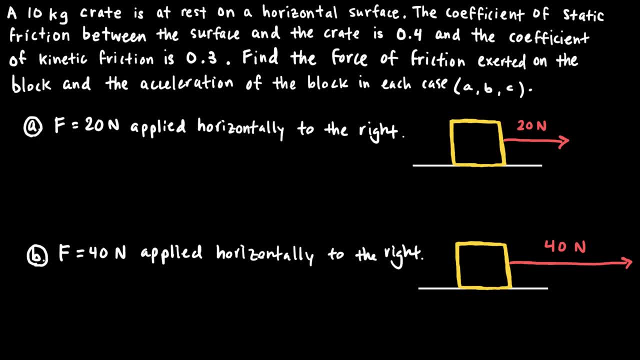 And if the force is anything equal to or less than that maximum value, then the block will remain at rest, And so the way that we determine what that value is is we write the equation: the force of friction, the force of static friction. 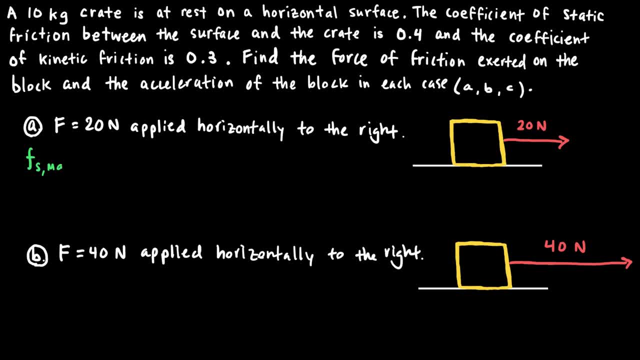 and really that maximum value of static friction is given by the coefficient of static friction times the normal force, And so in this case we do have a 20 N force that's acting to the right, but there's also the weight of the block, which acts down and is equal to mg. 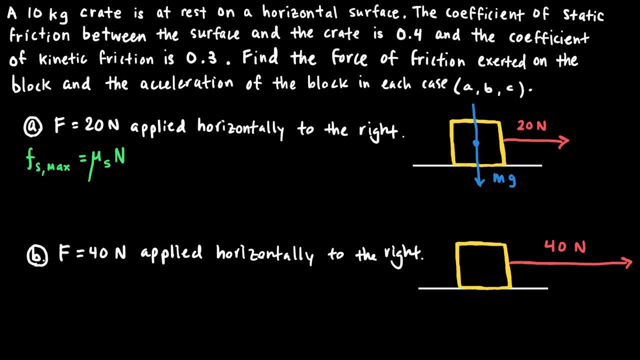 and then a normal force, which is equal and opposite, pointing upwards, which I'll label N, and then, because this applied force is to the right, the frictional force would point to the left And in this case we're not sure what kind of friction it is. 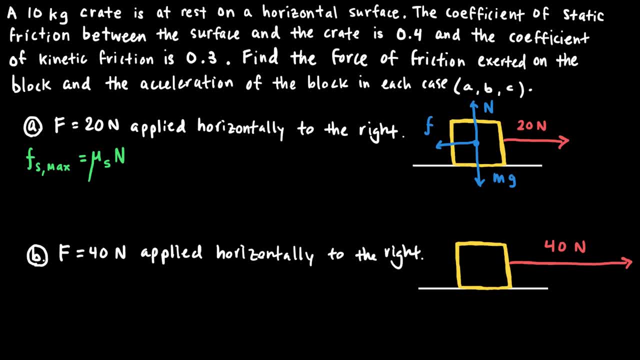 but we are trying to determine what is that maximum value of static friction which can be calculated using the coefficient of static friction and the normal force. So in this case the coefficient of static friction was given to be 0.4, up above in the problem. 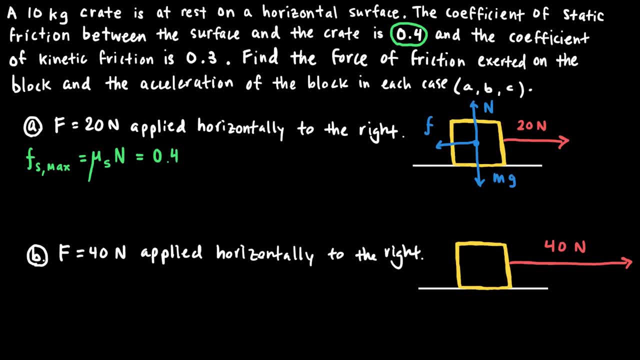 and the normal force is equal to the weight, which would be the 10 kg mass multiplied by 9.8.. And so the maximum value of the static frictional force is about 30 N. And the reason why that's important to understand. 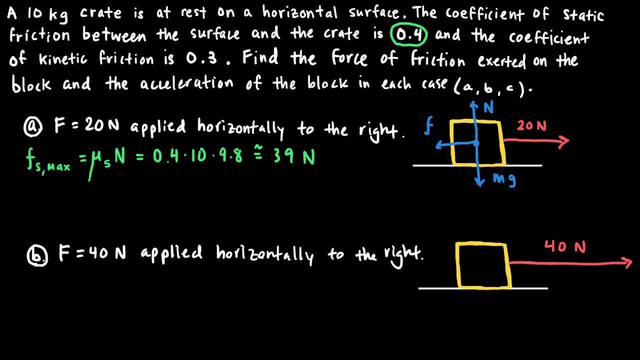 is applying a 20 N force is a force that is less than 39 N, which means the block is not going to move, And, in fact, if I applied a force of 38 N, the block would still not move. And so, in this case, because the applied force 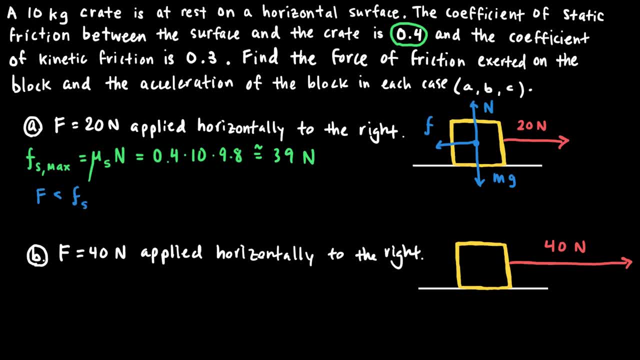 is less than the maximum value of the static friction, the acceleration of the block will be equal to 0.. The acceleration of the block is 0 because the force that is being applied is not enough to overcome the static frictional force that is possible between these two surfaces. 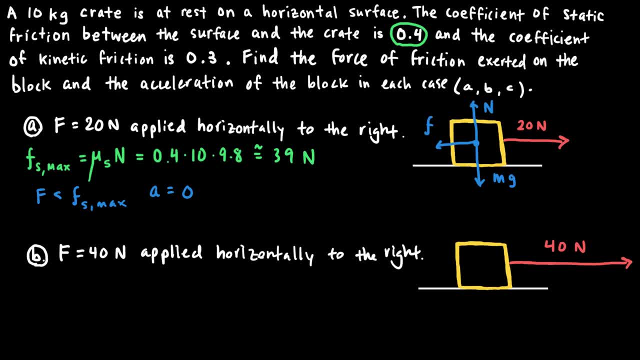 Now I still have not calculated the actual value of the frictional force between these two surfaces, and the way that I arrive at that value is pretty easy, Because the force is not large enough to make it move. the value of the force of friction. 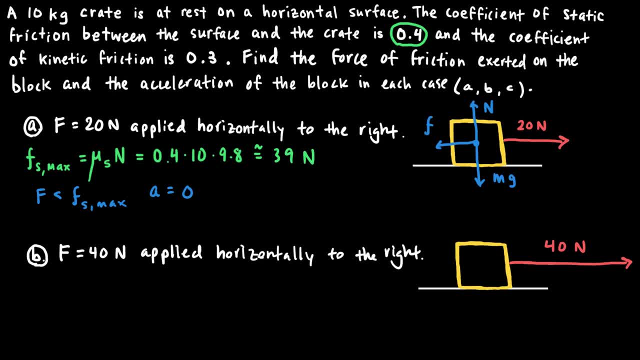 the force of static friction acting on this block is exactly equal to the force that's being applied, And so the acceleration is 0, and the force of friction that is acting on this block is 20 N At the end of the day. 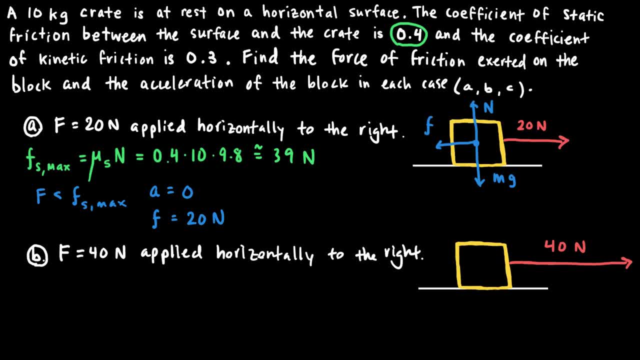 if we've now determined that this block isn't accelerating, it's not moving left or right, then we know that the 20 N force pointing to the right needs to be balanced by a force of equal magnitude in opposite direction, pointing to the left. 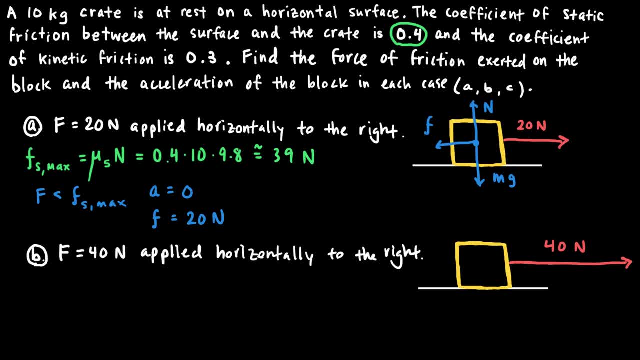 And so the force of friction acting on the block in case A is 20 N, and the acceleration is 0.. Now, clearly, in case B, something different is going to happen. Here the force that's being applied is 40 N. 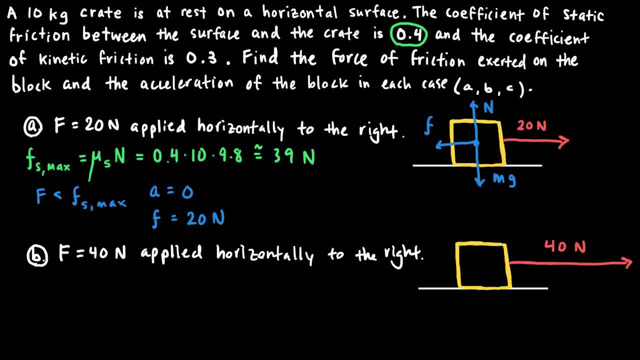 which means that the force that's being applied is greater than the maximum value of static friction, which means that when I apply that force of 40 N, the block should move. And so if the block is moving, if the block is sliding, 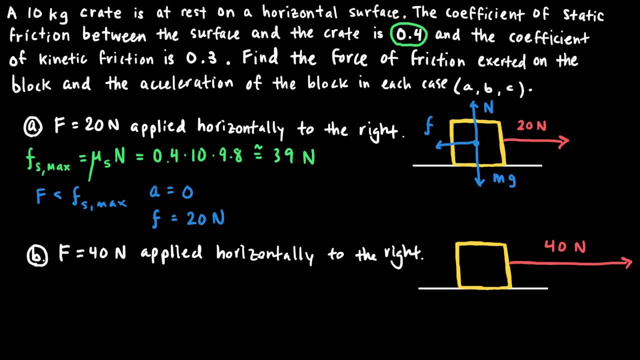 the way that I calculate the amount of friction that's acting on that block is no longer due to static friction, but instead kinetic friction, And so the value of the frictional force acting on that block should be given by the coefficient of kinetic friction times the normal force. 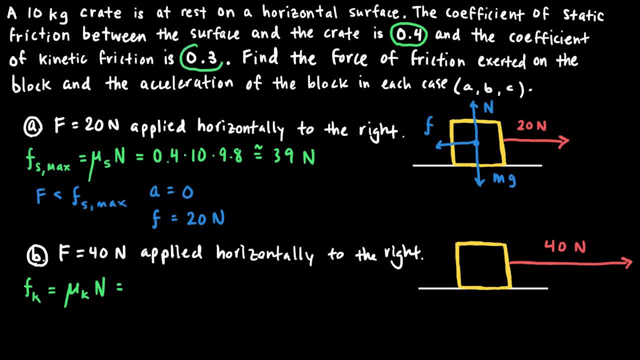 And here the coefficient of kinetic friction between these two surfaces was 0.3.. And once again, the normal force is the block's mass times gravity, 10 times 9.8.. And so, in this case, using the coefficient of kinetic friction, 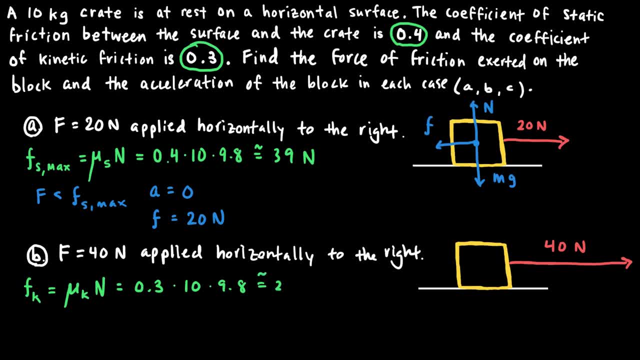 the value of the frictional force comes out to be about 29 N. So the frictional force is about 29 N And under the influence of that frictional force and the applied force, this block will experience an acceleration, But it's an acceleration due to the sum of those two forces. 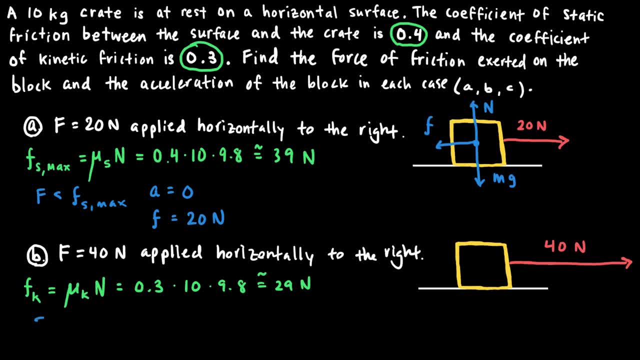 And so, in order to determine what that force is, I should write a Newton's second law equation which says: the net force acting in the x direction is equal to the object's mass times, the acceleration in the x direction. And I know that if I define the right direction to the right. 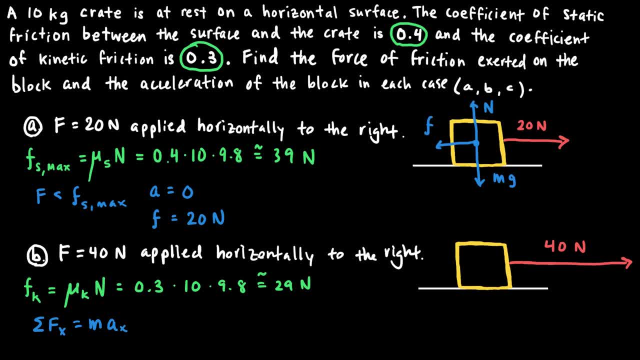 as the positive x direction. then the 40 N applied force, capital letter F is positive and the frictional force, lowercase f sub k, is a negative force because it points to the left right. This frictional force points to the left. 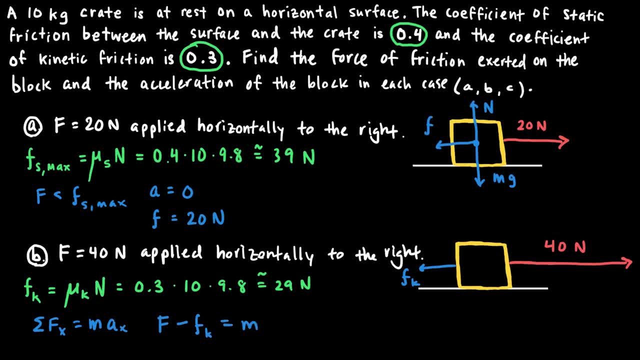 And that's equal to the object's mass, times the acceleration that is directed to the right, And so, in this case, the acceleration is given by 40 minus the frictional force of 29 divided by the mass of the block, which is 10.. 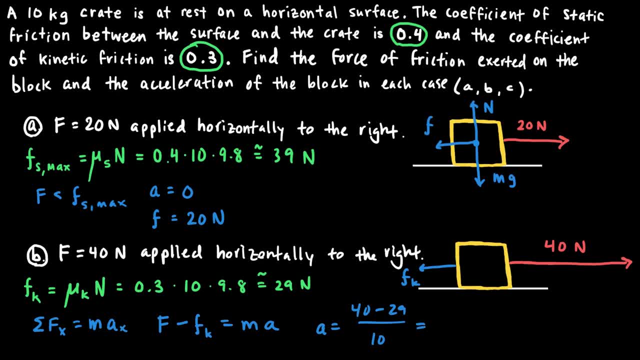 And so that comes out to be about 11 divided by 10, which is something near 1 m per second squared. And so the crate has a very moderate acceleration of 1 m per second squared. And so, comparing the two problems that we've done so far, 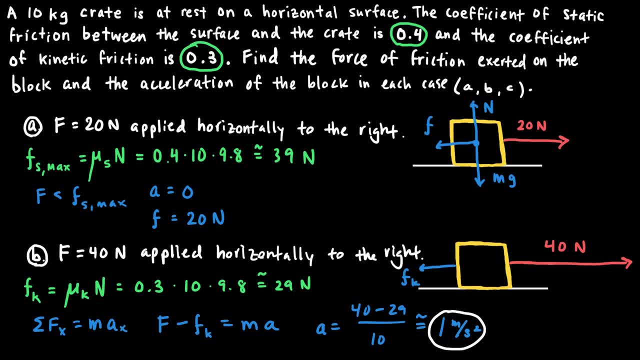 in the first case, we saw an example where the force that was being applied was less than the maximum value of static friction, in which case the block remained at rest and the frictional force was equal to the applied force. In the second case, we saw that the applied force 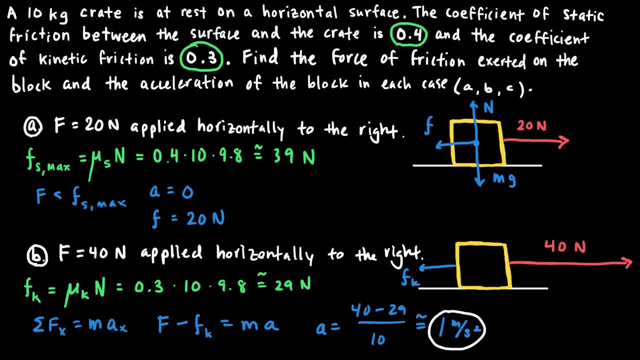 was larger than the maximum value of static friction, and so the block is no longer in equilibrium, It begins to accelerate, And so, as it slides, there's a force of kinetic friction which is less than that applied force acting on it, And it's due to the sum of those two forces. 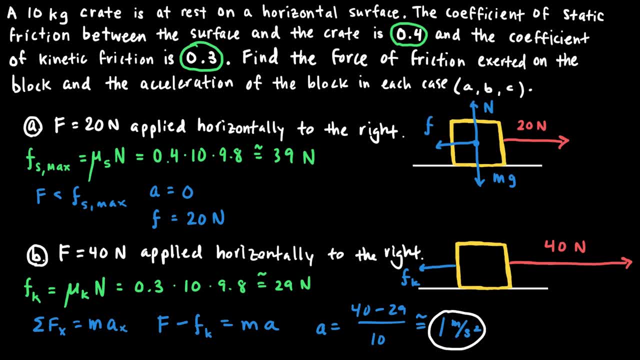 that the block experiences an acceleration to the right. And so so far for parts A and B. I know what the acceleration is and I know what the applied force of friction is on this crate In this last example, part C, 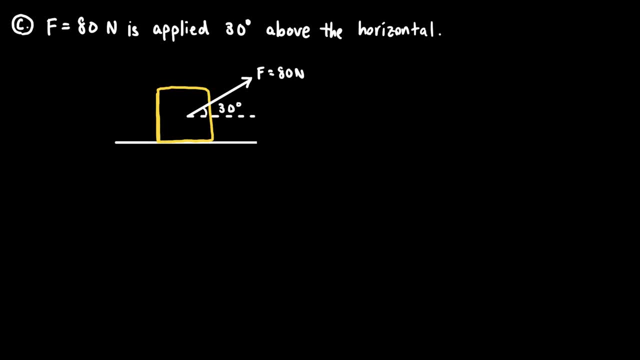 I'd like to have the force point in an angle so you can see how that adds a little bit of a challenge to some of the questions that we were dealing with in parts A and B. And so the first step really in those first couple of questions, 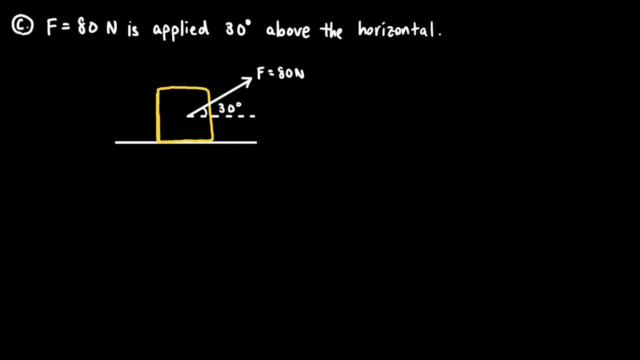 was to figure out whether or not the force that was being applied was larger than the maximum value of static friction. And so, if you remember, the maximum value of static friction, Fs max, was approximately 39 Newtons, And if you have a good intuition for 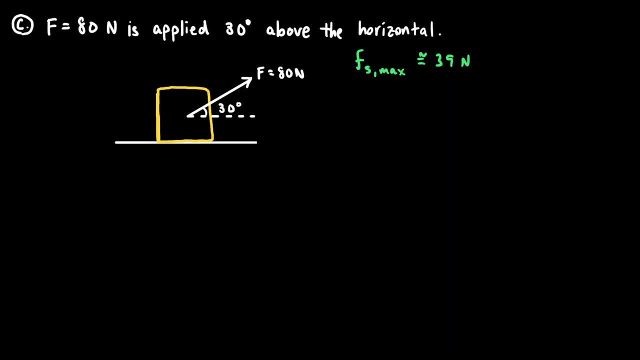 you know vector triangles and numbers, then you can probably look at this triangle and already tell me whether or not the force that would be responsible for the motion of this object is larger than 39 Newtons or not. But let's slow this down for a second. 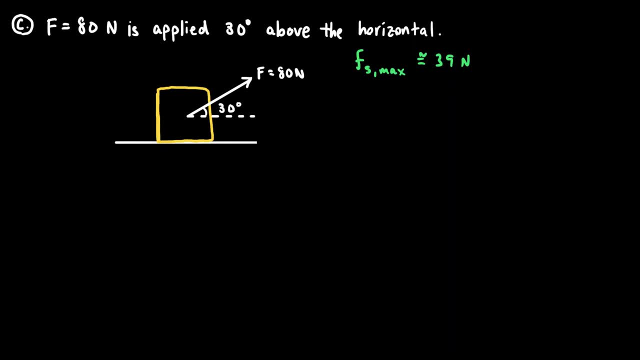 and think about the question that I'm trying to answer. If I'm going to determine whether static or kinetic friction is acting on this block, this crate, then what I really need to determine is: will the block move? But since the force is being exerted at some angle, 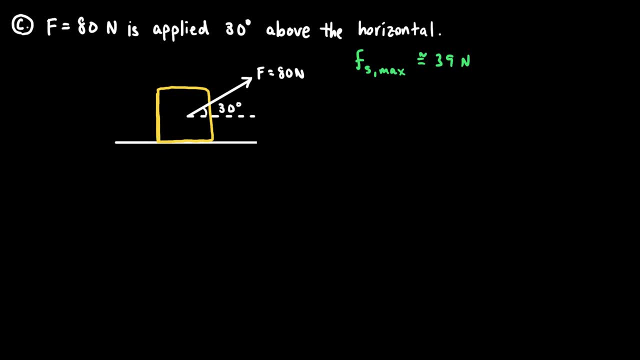 it's a little bit hard for me to determine that, And so, really, what I need to decide is: is the x component, is this horizontal component of the force that's being applied large enough to cause an acceleration of the block? And so I'll write Fx here. 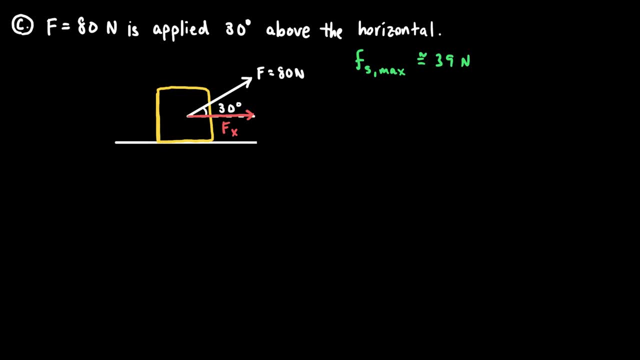 We'll refer to that as the x component of this force, And maybe there's a vertical component of this force that we can call Fy, And it's only the total force that's exerted at an angle that's 80 Newtons. 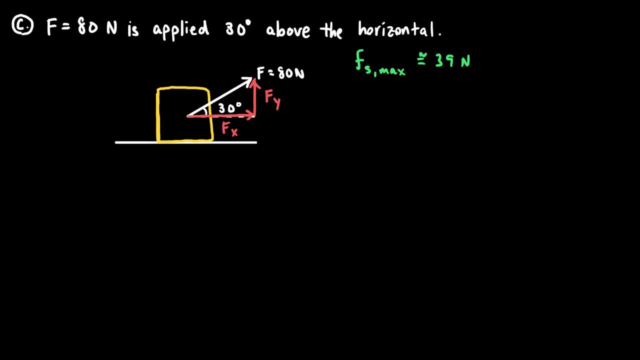 And if you remember your trigonometry, then you know that the x component of this triangle would be given by 80 cosine 30.. 80 cosine 30. And 80 cosine 30 comes out to be something like 69 Newtons. 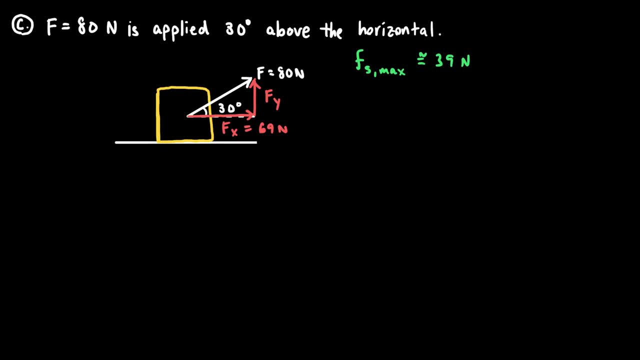 And if you tried to find the y component of this triangle, you would do 80 sine of 30 degrees and you would get 40. So these are the two components of this triangle. Now, if you think back to how we calculated the maximum value of static friction, 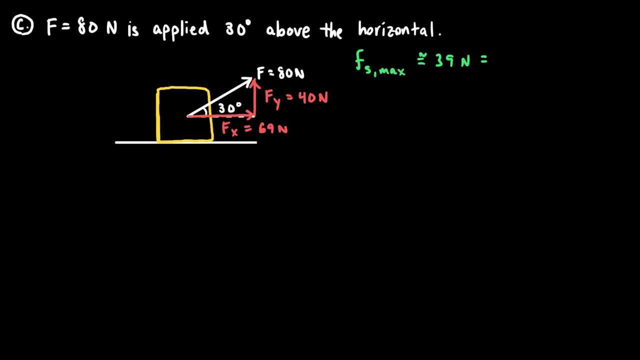 that 39 Newton force. you'll remember that we used the coefficient of static friction and the normal force. And now let's think about what happens to the normal force when I apply a force to the crate, that is, to the right and up The other forces acting on this crate. 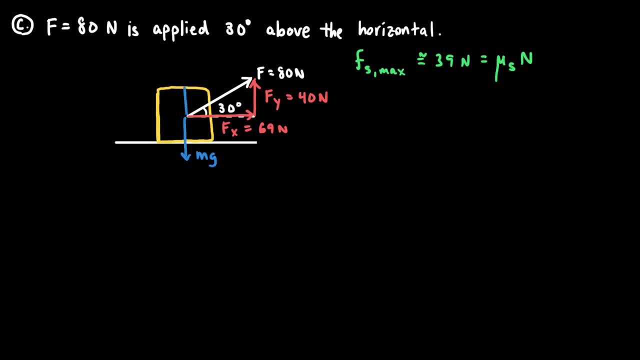 are the weight which points downward and the normal force which points up, And I want you to think of, instead of having this crate just sitting on the ground, I want you to imagine it sitting on a scale that measures mass, And imagine pushing down on the crate. 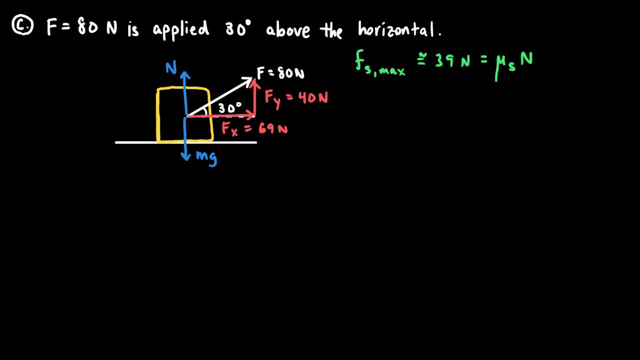 and seeing that the mass read by the scale would be greater. And imagine lifting up on the crate and seeing that the mass read by the scale would be less. And that scale? what it's really measuring is the amount of force that it has to apply. 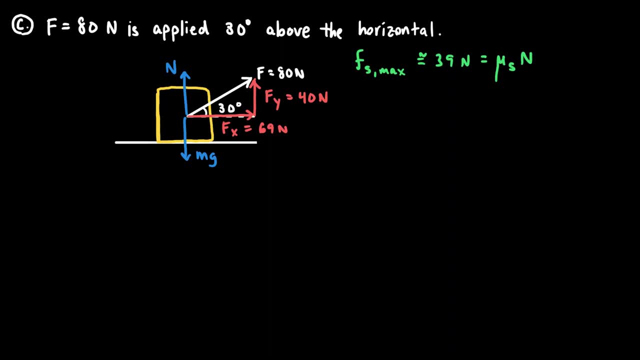 in order to lift you up. And so when I apply a force like this 80 Newton force, that's 30 degrees above, the horizontal part of that force is simply pushing to the right. It's pushing to the right in the same way. 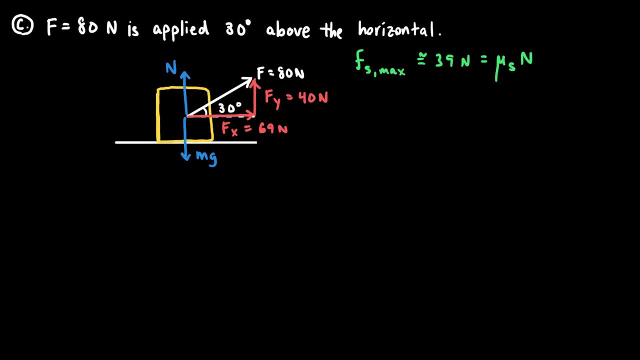 that those other applied forces push to the right. But a component of this force- Fy, 40 Newtons of this force- is pushing up, pulling up on this crate. And when that component of that force pulls up on the crate, 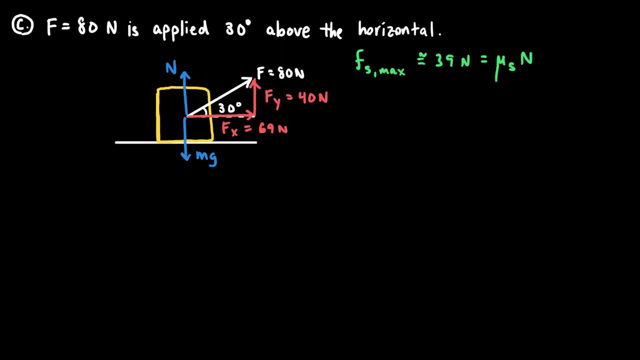 the ground doesn't have to do as much work in order to hold that crate up. What I'm trying to say is that the vertical component of this 80 Newton force lessens the normal force. It decreases the normal force. In fact, if we were to draw a separate free body diagram. 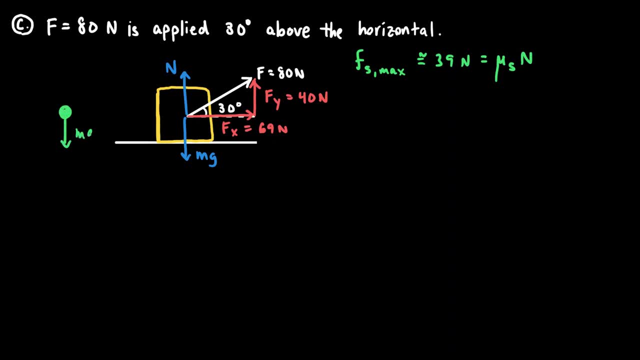 we would see that the weight points down Mg, and there are actually two forces that point up: the normal force and Fy, And in order for the block to remain in equilibrium, it's the normal force plus Fy that have to balance out the weight of the block. 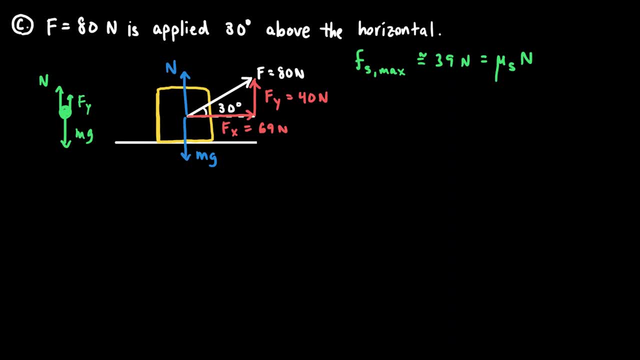 And so the more I pull up on the block, the less N becomes, And so in this instance, if I wanted to do this problem carefully, really, what I should do is calculate a new value of the maximum static frictional force, And that would be the value of static friction. 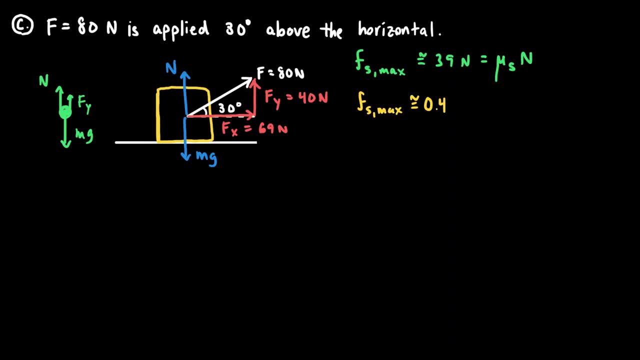 which was for the coefficient, which was 0.4, times the new normal force. And in order to find that new normal force, I think it's going to involve a little bit of calculation. I know that in the y direction. 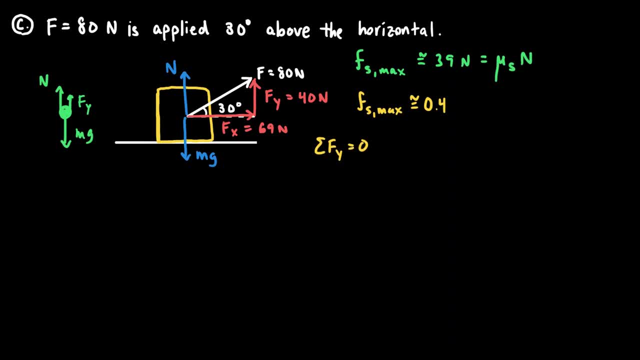 the forces must add up to 0, because the block is remaining at rest, It's not accelerating upward, And what that means is that the normal force and the vertical component of the applied force, which point up and are positive, minus the weight of the block. 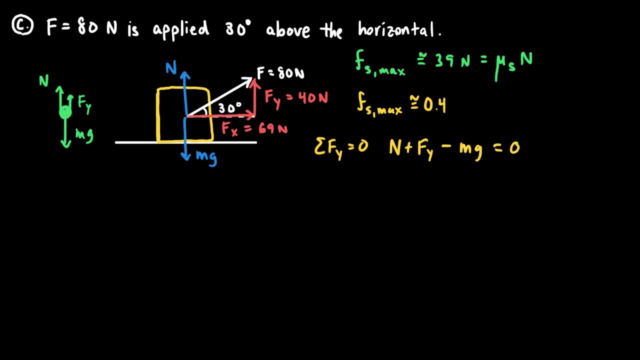 should add up to 0.. Therefore, the normal force is given by the weight minus Fy. And if the mass of the block was 10 kilograms and the acceleration due to gravity is 9.8, and the vertical component of the force was 40,, 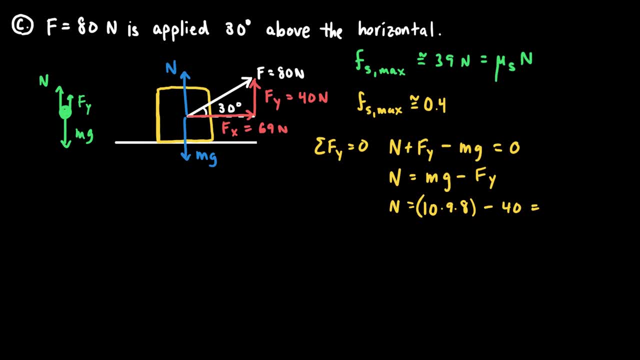 then 9.8 times 10 is 98, minus 40 is 58 newtons, And so the new normal force is 58 newtons. So going back up above, I should be able to calculate a new value for the maximum static frictional force. 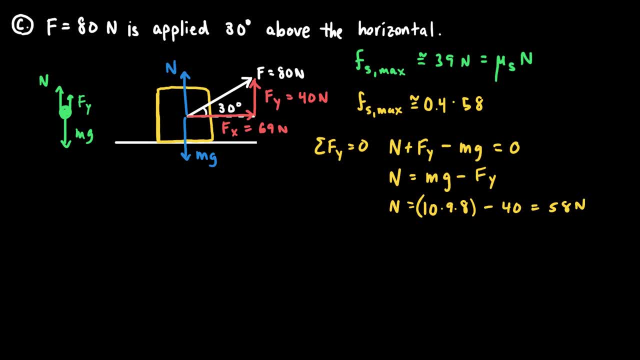 And that would be 0.4 times 58, which is about 23.2.. So let's just say it's about 23 newtons. And so, notice, due to the upwards pulling from that applied force which lessens the normal force, 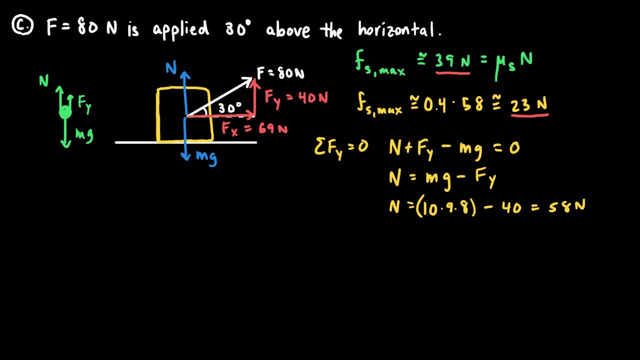 the maximum value of static friction was also lessened. I don't think that what I've done is immediately required in order to solve this problem. Originally, the x component was 69,, which was much larger than the maximum value of static friction. 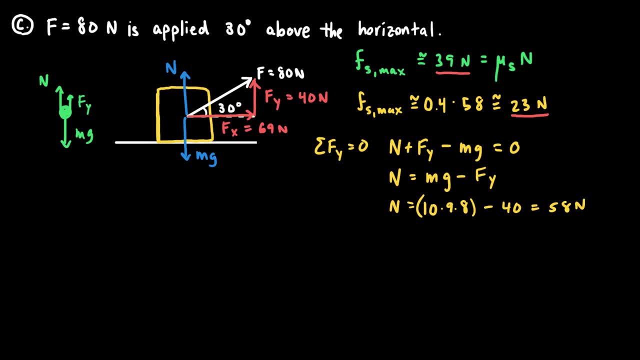 And by pulling up on the block that's only going to lessen the maximum value of static friction, And so I should have known from the onset that this calculation was not necessarily required. In fact, I knew already that it had to be kinetic friction acting on the block. 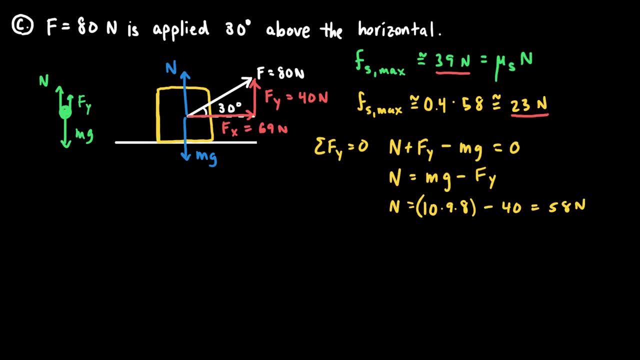 because I knew it was going to slide, because 69 is already larger than 39. And so, to go back to the problem, I know now that the force of friction acting on the block is equal to the coefficient of kinetic friction times the normal force. 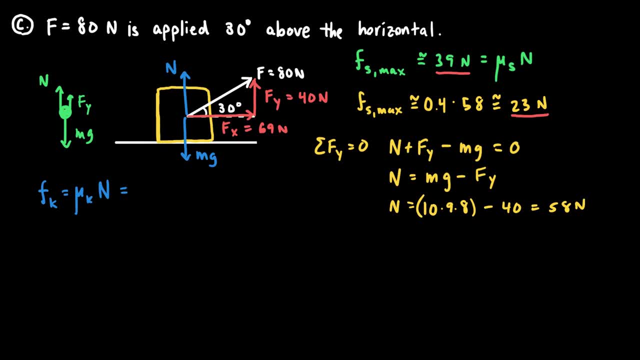 And so I guess I was going to need the value of the normal force anyway, since I would need it for this calculation. And so the coefficient of kinetic friction is 0.3, and the value of the normal force is 58 newtons. 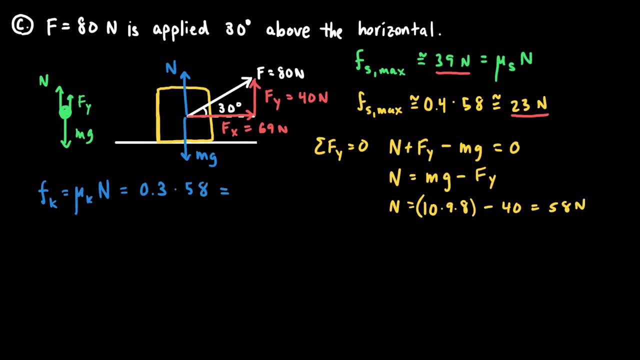 And 0.3 times 58 comes to be about 17 newtons. And so what this means, to boil it down into its simplest terms, there is a 69 newton force pointing to the right and there is a 17 newton force. 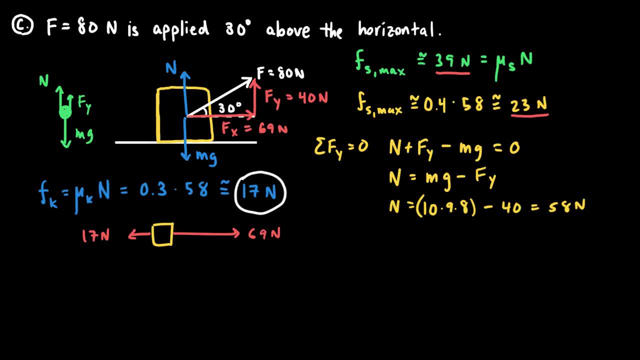 pointing to the left. The x component of the applied force to the right and the force to the left is the force of friction And again it's due to the sum of these forces in the x direction that gives us the acceleration in the x direction. 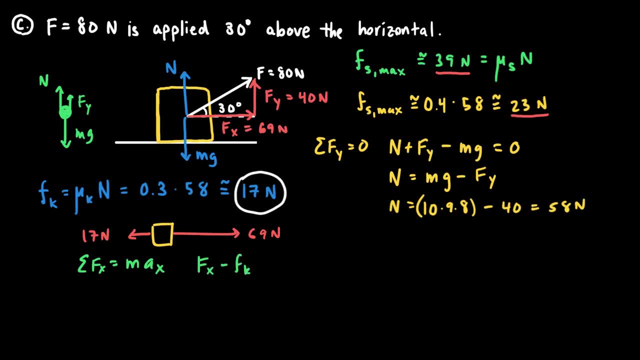 So really f minus the frictional force, that kinetic frictional force is equal to the object's mass times, its acceleration, And so we've already determined that kinetic frictional force, and so we can simply say 69 minus 17 divided by 10. 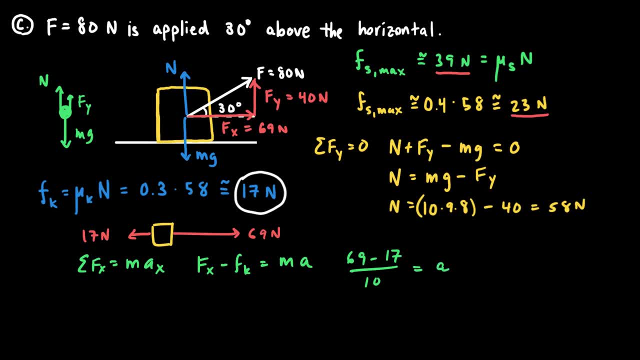 would be equal to the acceleration of this block, And I believe that comes out to be something close to, maybe a little bit north of 5 meters per second squared, And so this is quite a large acceleration, which seems to make sense, because when I look at the free body diagram, 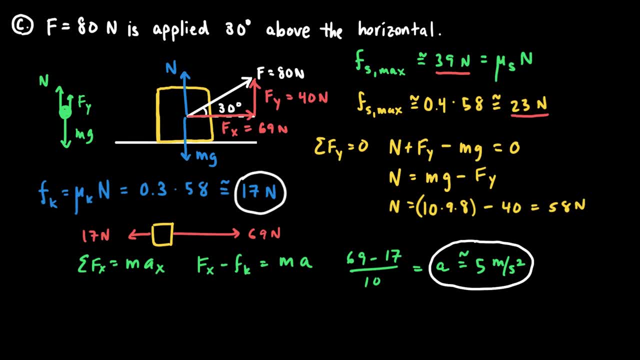 the 69 newton force is much larger than the 17 newton force. Here the value of the force of kinetic friction was 17 newtons, and if you refer back to part b, we found a force of kinetic friction that was only about 29 newtons. 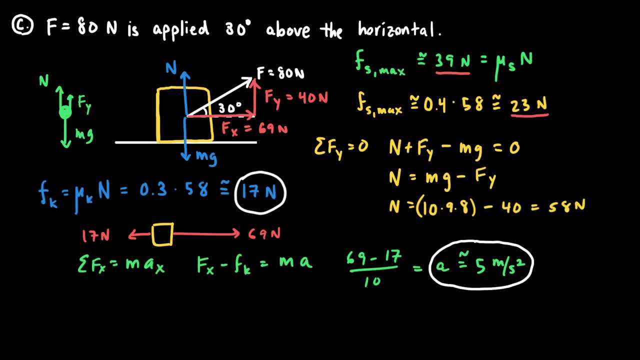 And so there's a big difference there. Now, typically we say: no matter what force I apply, the moment I get that crate moving, the force of kinetic friction would be the same. And that would be true if we weren't comparing two different cases. 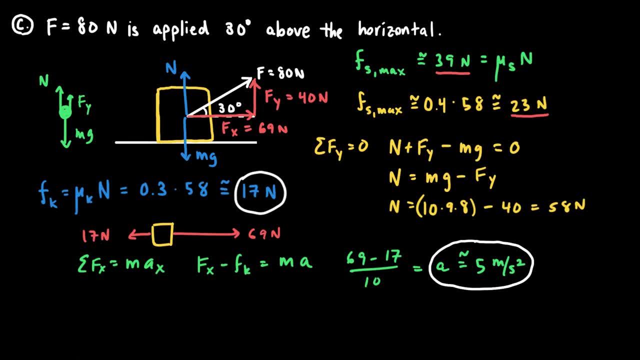 where the normal forces were different in each case. And so here, in addition to understanding some of the problem solving things that I mentioned- how to determine if it's static or kinetic friction- I think one big thing comes out of the third part of this problem.